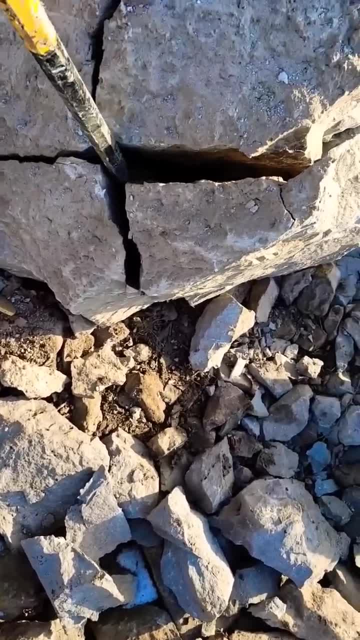 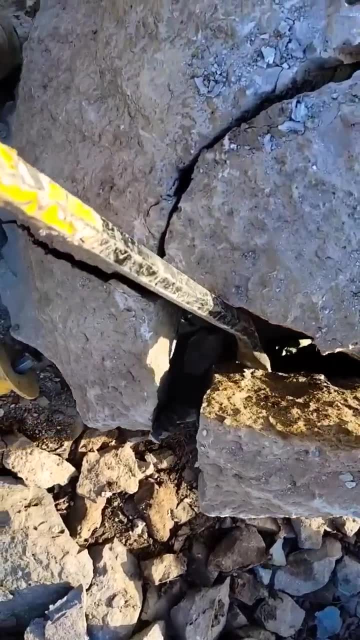 oh yeah, okay, hold on, look at that. okay, right here. no pockets yet, yep. 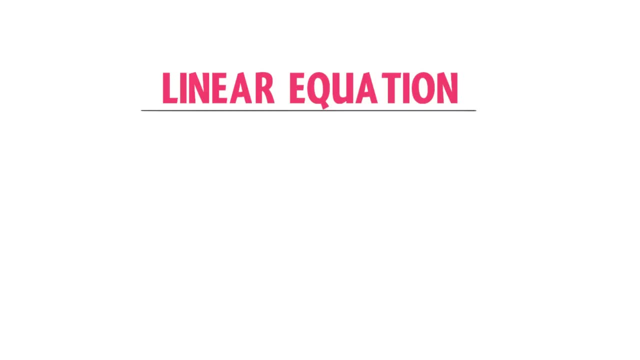 Linear equation. In this lecture we will discuss about linear equation in one variable and linear equation in two variables, or first degree equations. If I write, 4x plus y is equal to 6.. In this equation there are three terms: 4x, y and 6.. The x and y are known as 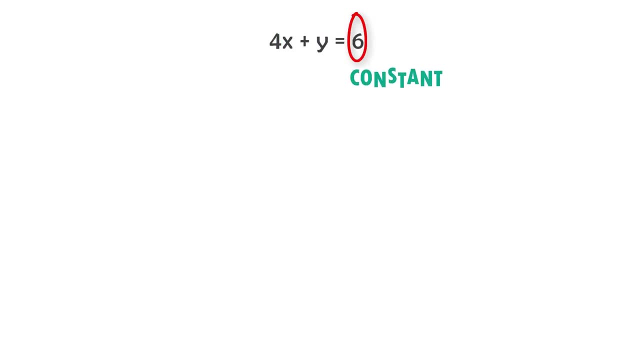 variables, While 6 is the constant and 4 is the coefficient of variable x, The highest power of the variable x is 1 and the highest power of the variable y is also 1.. Hence, all the variables in this equation have the highest power 1.. Therefore, this equation is known. 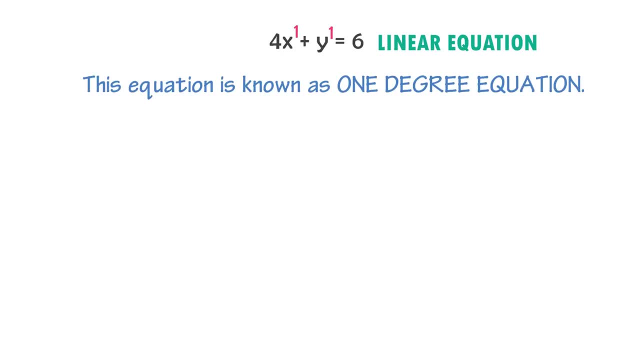 as a one-degree equation or linear equation. Let me give you another example: 2xy plus 5 is equal to 10.. This equation has also three terms: 2xy, 5 and 10.. The term 2xy is considered. 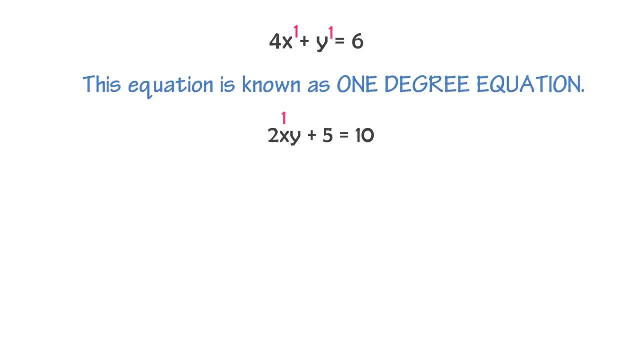 as a one term. The power of x is 1 and the power of y is also 1.. Hence 1 plus 1 is equal to 2.. Thus the highest power of this equation is 2.. Therefore it is not one-degree equation. 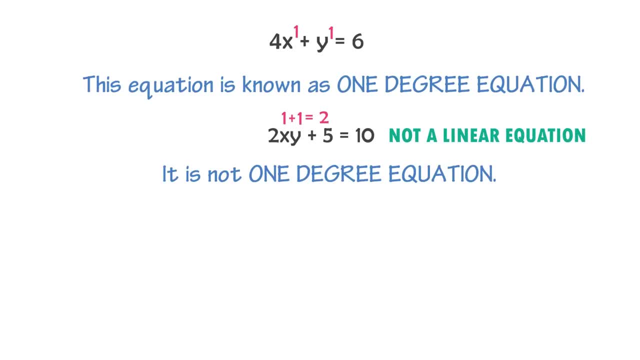 Hence it is also not a linear equation. Now again, if I write 4xy plus 4yz is equal to 80. In this equation x plus 2yz is equal to. Now again, if I write 3x plus 4yz plus xz is equal to 80.